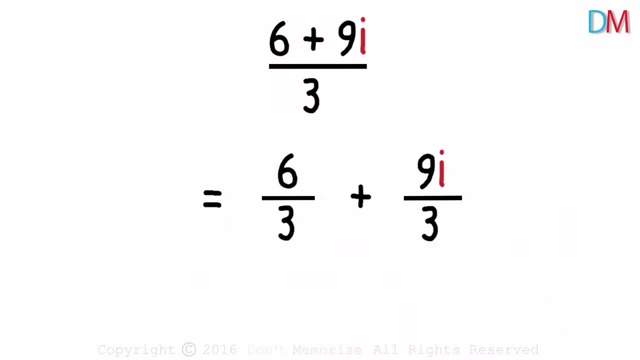 We get 6 over 3, plus 9i over 3. That will equal 2 plus 3i. So dividing a complex number by a real number is easy. How about dividing a complex number by an imaginary number, Say 6 plus 9i over 4i? 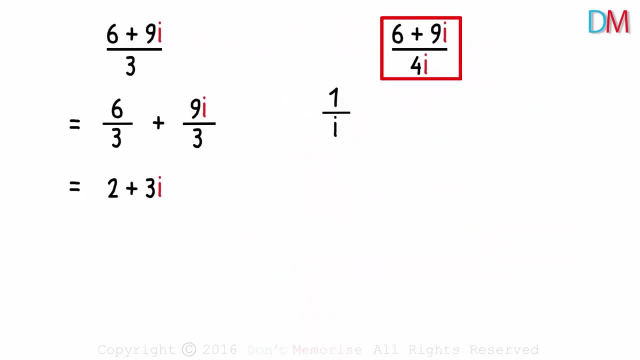 Before we solve this, let's understand what 1 over i means. Not very comfortable having i in the denominator. So how can we get rid of it? It's easy: We can multiply the numerator and the denominator by i. That gives us i over i squared. 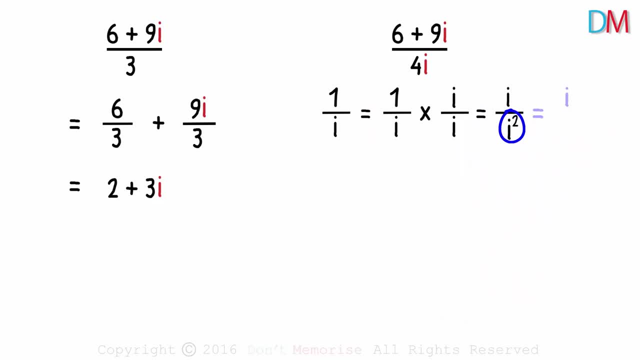 And i squared is nothing but negative 1.. And i over negative 1 is nothing but negative i. So 1 over i is equal to negative i. Now let's proceed with the problem. Dividing 6 plus 9i by 4i is equal to 1 over i over 3.. Now let's proceed with the problem. Dividing 6 plus 9i by 4i is equal to 1 over i over 3.. Now let's proceed with the problem. Dividing 6 plus 9i by 4i is equal to 1 over i over 3.. 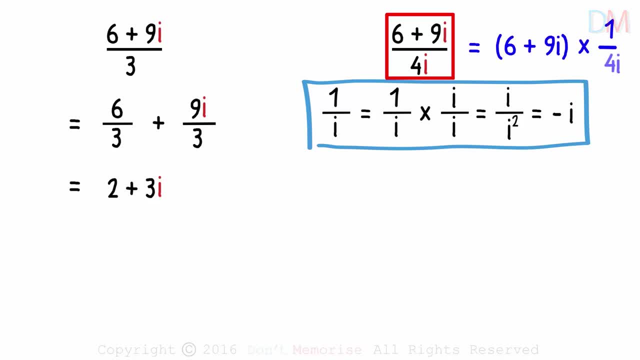 Now let's proceed with the problem. Dividing 6 plus 9i by 4i is equivalent to multiplying 6 plus 9i with 1 by 4i, So this will give us 6 over 4i plus 9i over 4i. 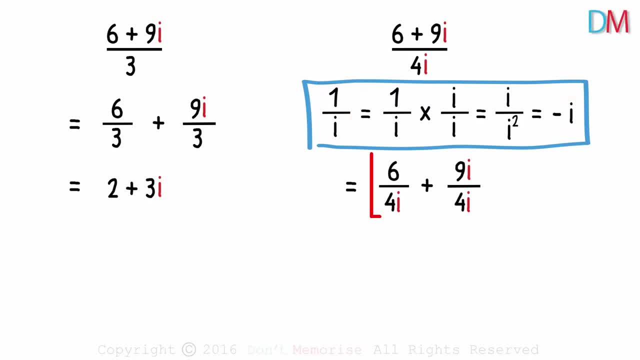 As we saw that 1 over i is negative i, this can be written as negative 6i over 4 plus 9i over 4i. Simplifying this will give us negative 3i over 2 plus 9 over 4.. 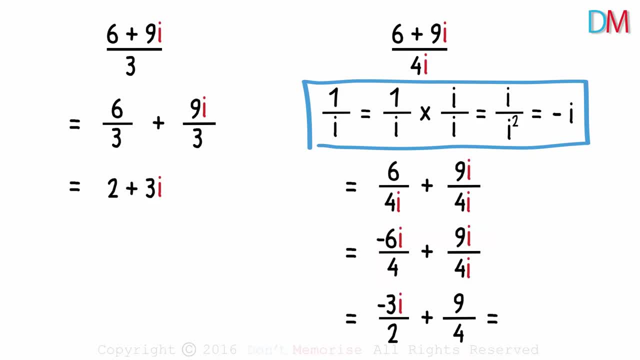 As we write a complex number with the real number first is 9 over 4 minus 3i by 2.. So dividing 6 plus 9i by 3 gives us 2 plus 3i, And dividing 6 plus 9i by 4i gives us 9 over 4 minus 3i by 2.. 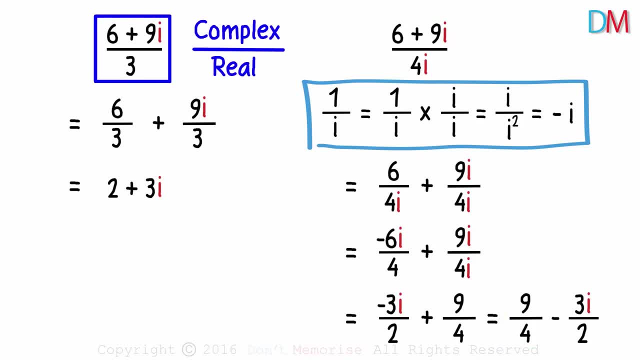 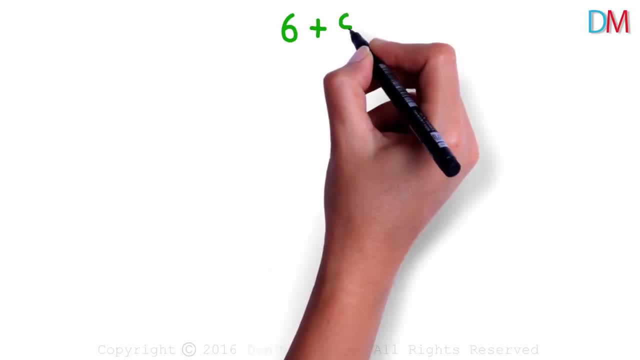 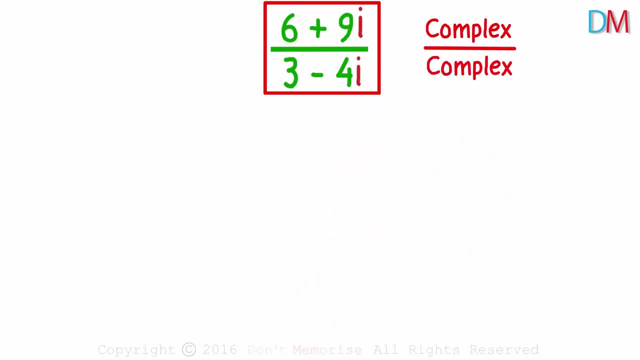 Clearly, dividing a complex number by a real number or an imaginary number is quite easy. How about dividing 6 plus 9i by 3 minus 4i? This is a case of a complex number divided by a complex number. Is this easy? 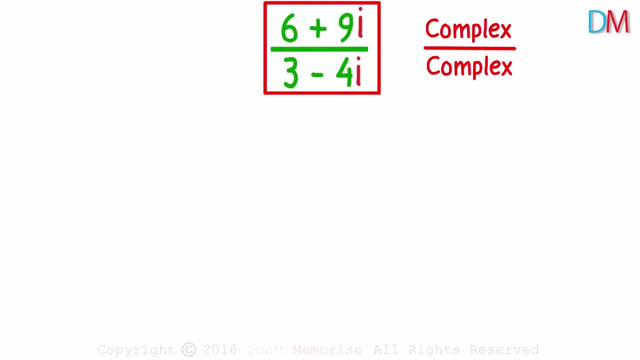 Before we go ahead with the solution, I want you to think about how we can approach this. Just give it a thought. Well, when I had seen a similar example in school, I had no idea how to proceed. So don't worry, this may not appear to be simple. 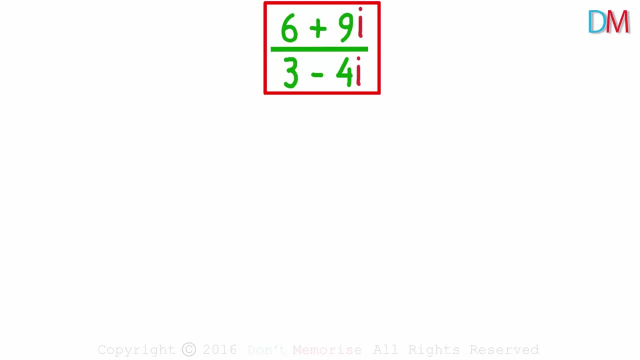 but there is a way out. Just remember one thing: in general, None of us like having i in the denominator. It just doesn't look perfect. So can we get rid of i in the denominator without changing the value of the overall expression? 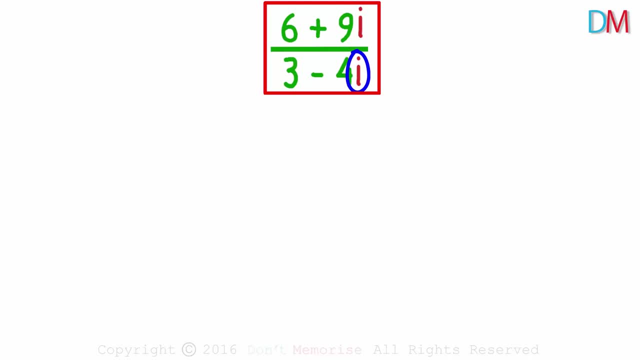 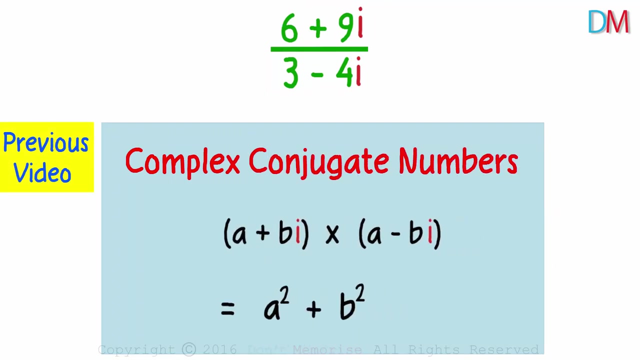 This was a big hint. Think about how we can proceed. Do you recall the discussion regarding complex conjugate numbers? in our previous video, We had observed that multiplying a complex number, a plus b, i with its complex conjugate a minus b i, resulted in a squared plus b squared. 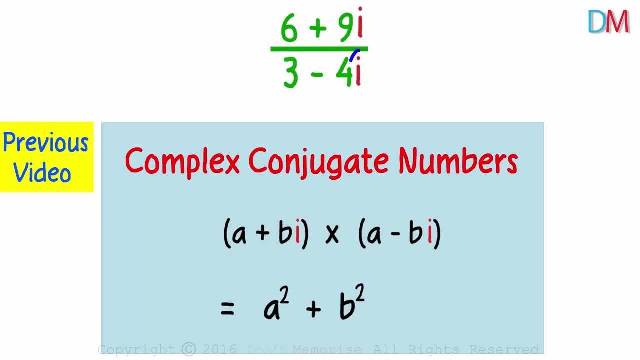 which is a real number. So to get rid of i in the denominator we need to multiply it with its complex conjugate, And to keep the value of the fraction unchanged we will also have to multiply the numerator with the same complex conjugate. 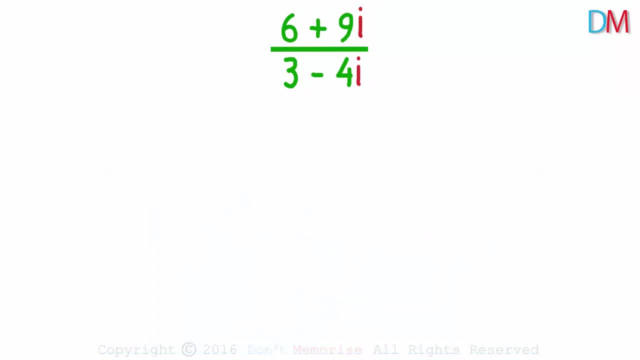 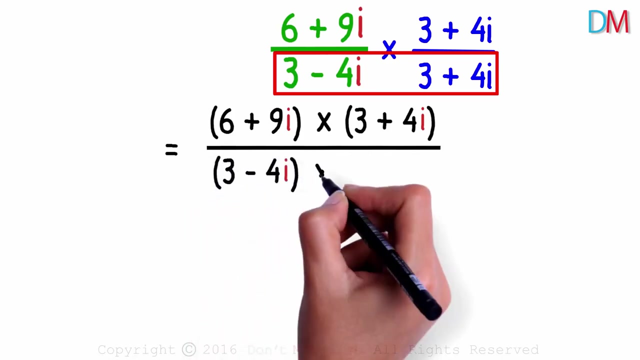 So we multiply the numerator and the denominator by the complex conjugate of three minus four i, which is three plus four i. This makes the numerator as six plus nine i multiplied by three plus four i, and denominator as three minus four i multiplied by three plus four i. 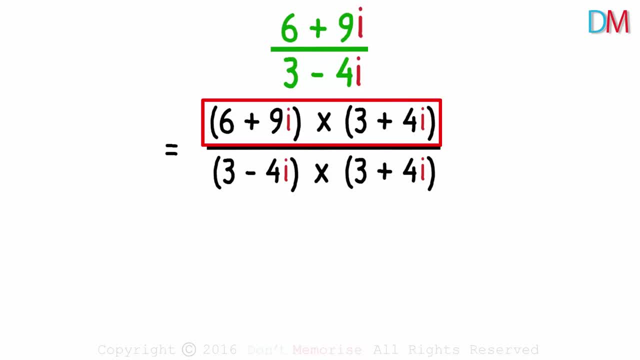 The numerator here becomes a classic case of multiplication of two complex numbers And the denominator is a case of multiplication of complex conjugates. Let's simplify the numerator first. It will equal six plus nine i multiplied by three plus six plus nine. i multiplied by four. i. 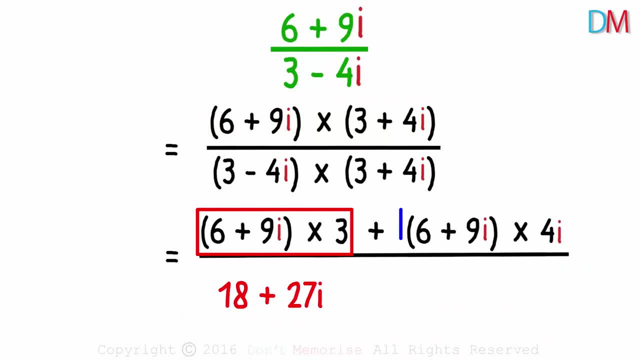 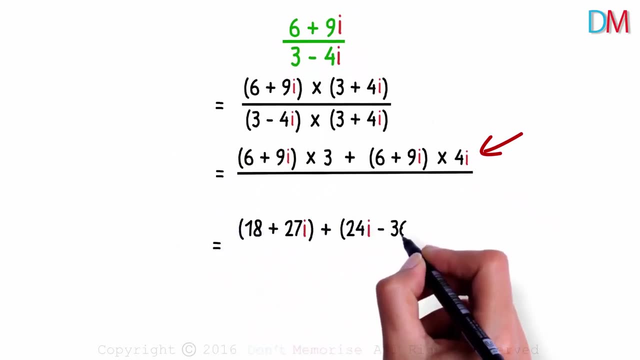 This will give us eighteen plus twenty-seven i, and this gives us twenty-four i plus thirty-six times. i squared, That will be twenty-four i minus thirty-six. Hence the numerator is addition of eighteen plus twenty-seven i and twenty-four i minus thirty-six.